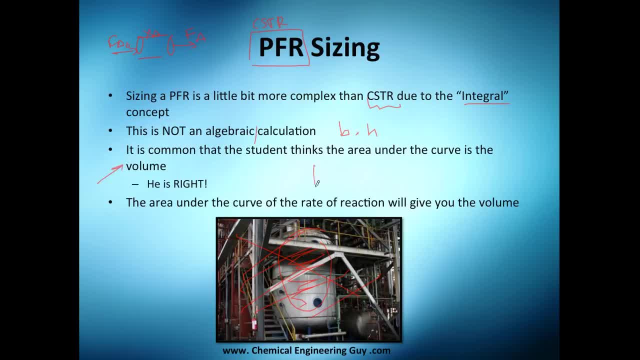 And, as I told you before, many students I give you or I give them this and they tell me that the volume should be the area under the curve. here, And they are actually right- For PFR, it is the factor that, independent of how the shape is, the area under the curve is the volume. 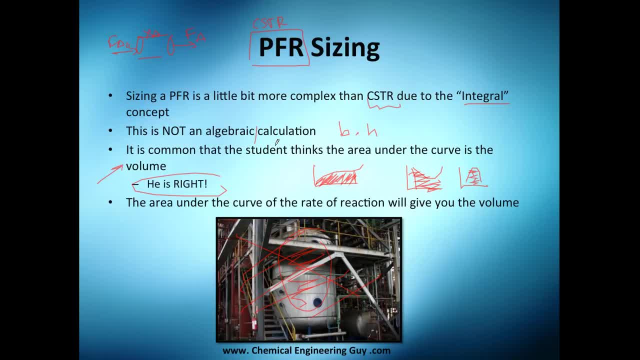 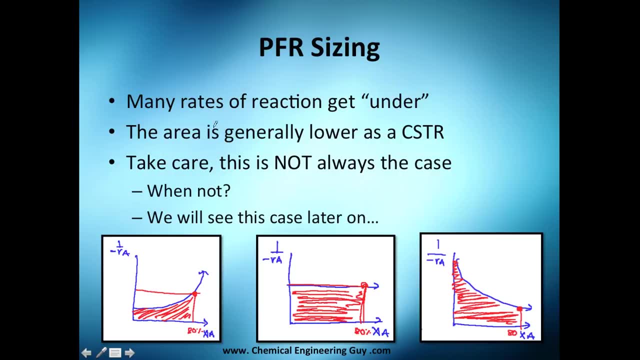 So that will help you a lot, and normally that means we're going to do integrals. So, independent of the type of rate of reaction we will have to calculate these areas under. In general the areas are lower than continuous hang reactors. That's not always the case Actually. we're going to see later. 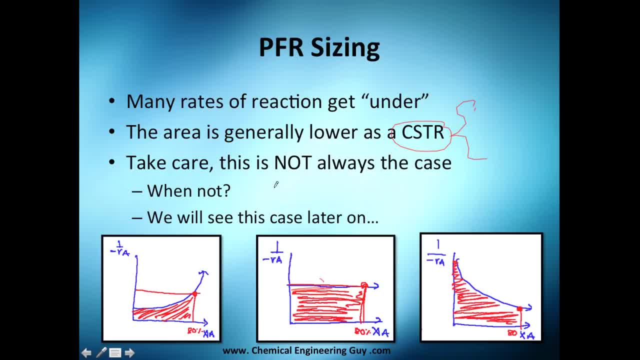 when it's not the case. When not, yes, let me show you first case, This one here: if I calculate a PFR will be the area under this, and you know that if I used to calculate a CSTR, it will be this here also included. So you can see that this. 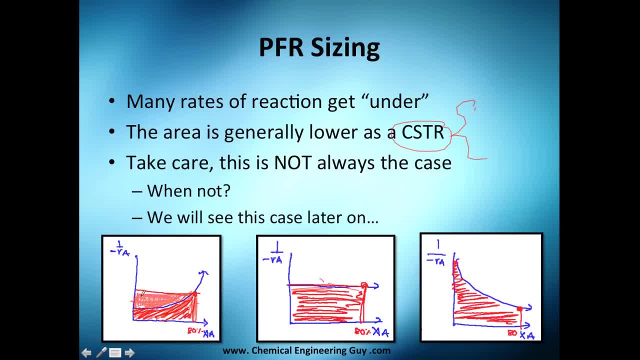 is like a waste of space. if you use another reactor, This one is actually the same. The volume of a CSTR will be the same volume as a PFR, due that this is actually a rectangle. So let's say we force the rectangle so it's the same volume. And final but not least, and actually this is: 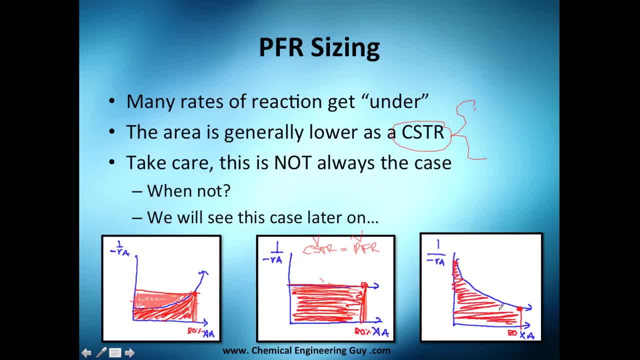 the only case in which the volume of a CSTR will be, let's say, large- how to say it? more than that is whoops, wait for it. yeah, here it's. here You can see that the CSTR value will be only here, this little rectangle, And the PFR is wasting all. 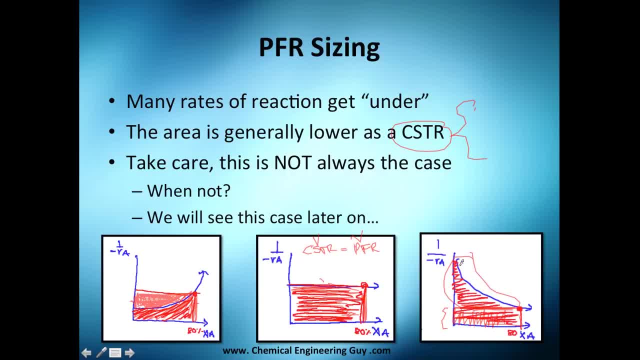 these sides. So well, not actually wasting, because without it you will not be able to achieve that conversion, What I mean? that you could be having a reactor which does not require it. So taking away this, you are done. You know now when are the cases, but just.